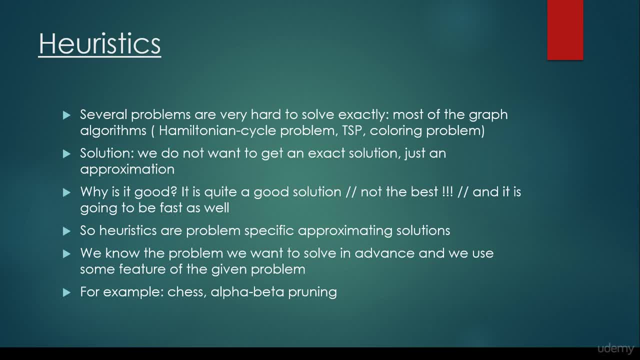 problem. All of these problems are very complex. These are the so-called MP problems- non-deterministic polynomial problems- And the solution is that we don't want to get an exact solution, we just want to end up with an approximation of the solution. Why is it good? 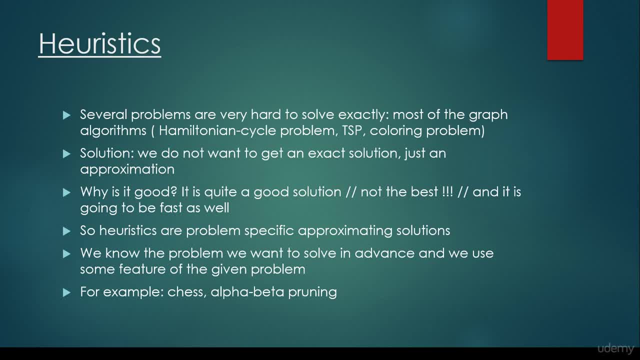 Because it is quite a good solution. Okay, it's not the best, but it is approximately the best. And it's not the best but it is approximately the best And, on the other hand, it's going to be very fast. This is what we have been discussing for. 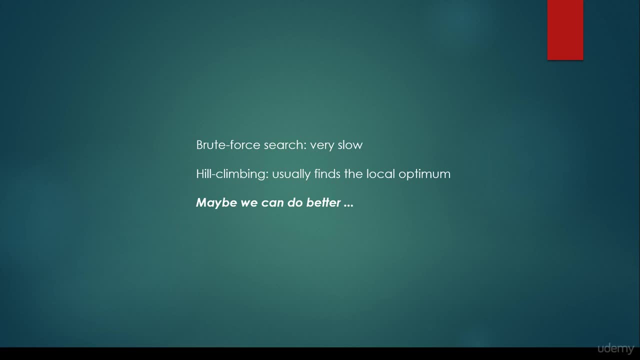 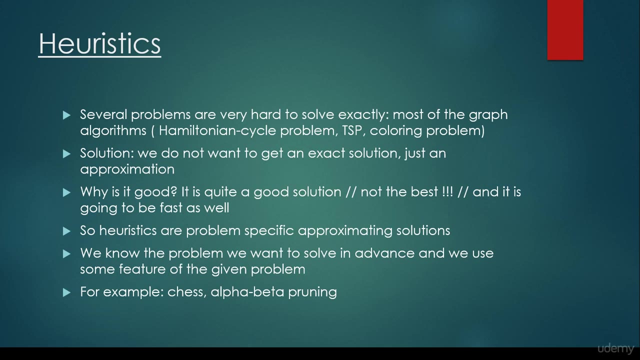 brute force search. that okay, it's going to find the best solution possible, but it's not going to be fast, It is very, very slow. Heuristic algorithm is going to find approximately the best solution- not the best one, but approximately the best solution- And, on the other hand, it's going to 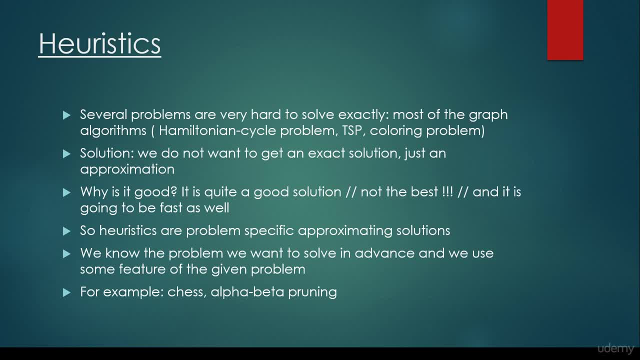 be fast. So heuristics are problem-solving algorithms and they're going to be very, very problem-specific, approximating solutions. It's very important that we know the underlying problem and we are going to construct the heuristic algorithm accordingly. We have already. 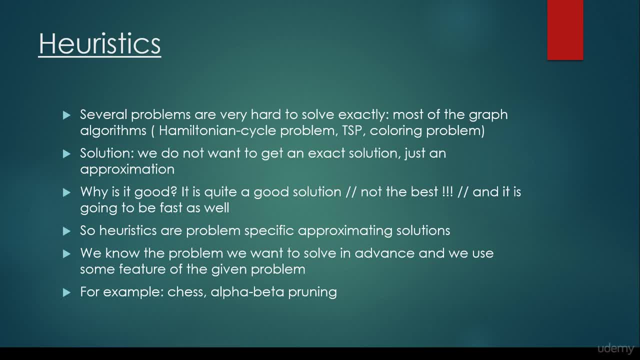 considered a heuristic algorithm. This is the so-called A-star search that we know for certain that we are going to do a search algorithm and we would like to find the shortest path on a given graph. So we know the underlying problem and we use some feature of that. 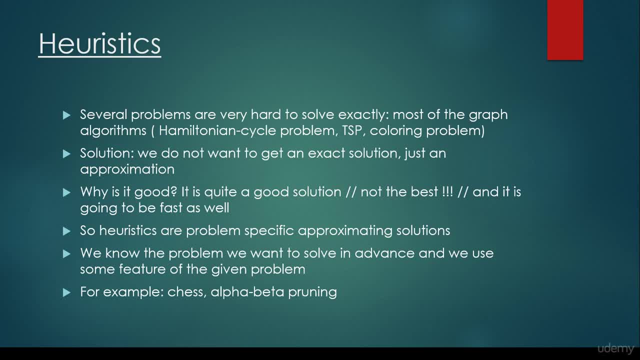 given problem. For example, chess or tic-tac-toe fell into this category and that's why the solution is going to be alpha-beta pruning. We are going to consider it in the next section. So solving tic-tac-toe and chess with the help of alpha-beta pruning is a heuristic algorithm. 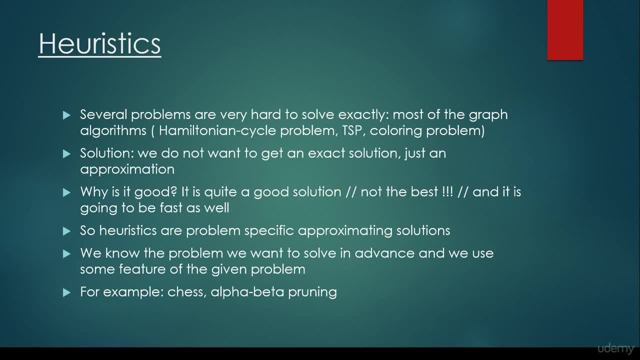 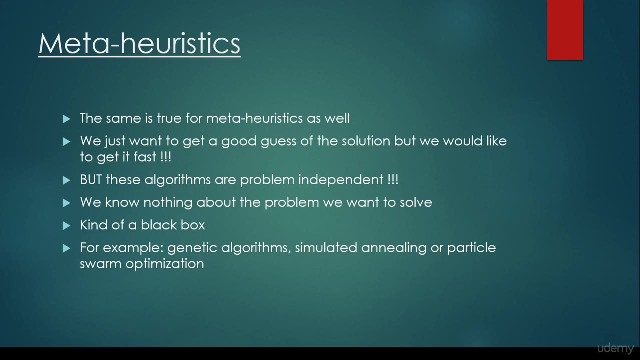 We know the feature of the given problem, and that's why we are able to construct the problem-specific algorithm, the so-called alpha-beta pruning. What about meta-heuristics? The same is true for meta-heuristics as well, what we have discussed. 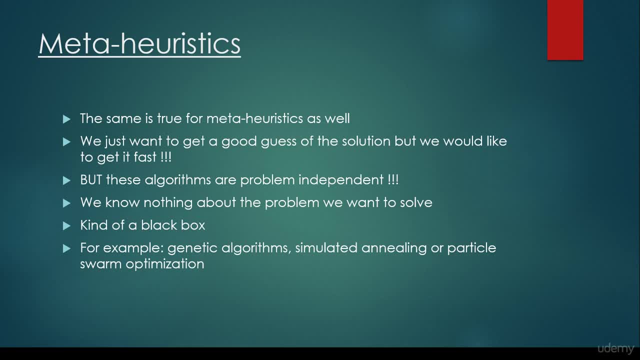 for heuristics. So we want to get a good guess of the solution, but we would like to get it quite fast. So that's why we are not able to use the brute force search, because it's not going to be fast. But these algorithms are problem-independent. It's very important that we don't know the 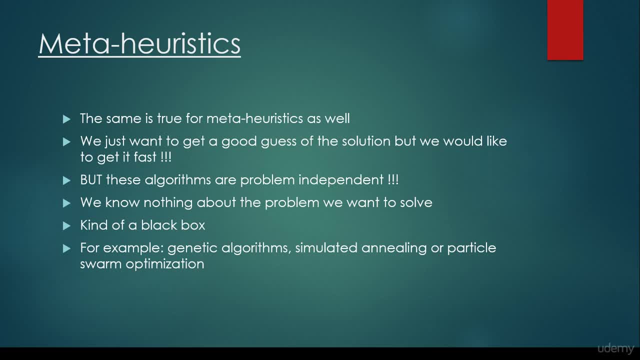 underlying features of that given problem. We know that the algorithm is not going to be fast. we know nothing about the problem we want to solve. it's kind of a black-box method. For example, genetic algorithms, simulated annealing or particles form optimization fell into this. 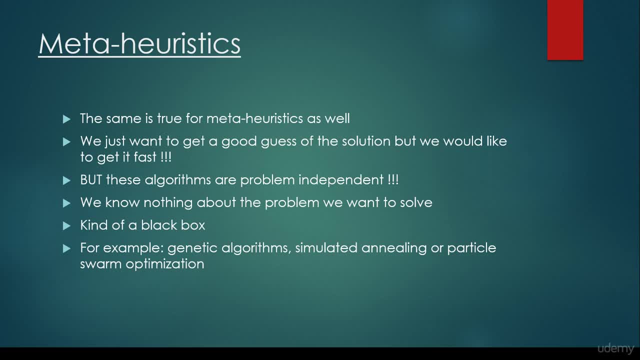 category. And okay, what does it mean? that we know nothing about the concrete problems? or it is problem-independent? It means that, for example, we are able to solve N-queen's problem with the help of genetic algorithms. we are able to optimize a given function. 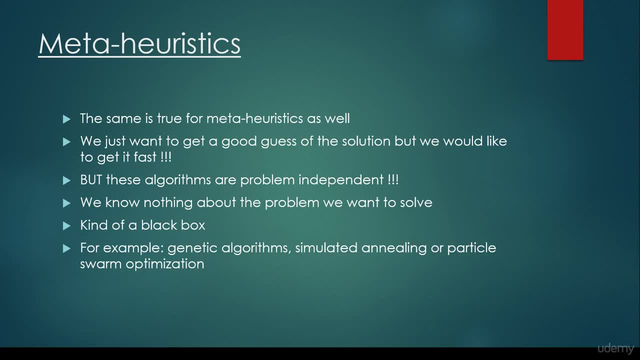 so we are able to find the minimum or the maximum value. we are able to solve graph algorithms such as the traveling salesman problem, and we are able to use the same approach for all these problems. We are not able to use alpha-beta pruning, for example, for solving traveling. 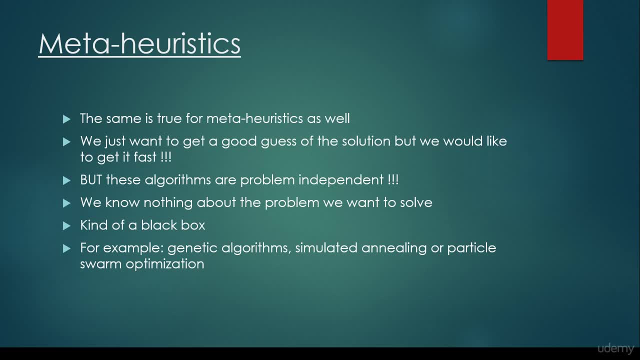 salesman problem, because alpha-beta pruning is used for chess or tic-tac-toe. That's why alpha-beta pruning is a heuristic algorithm. Genetic algorithms simulated annealing or particles form. optimizations, on the other hand, are meta-heuristic algorithms. We have the base theory and we are able to use it for several 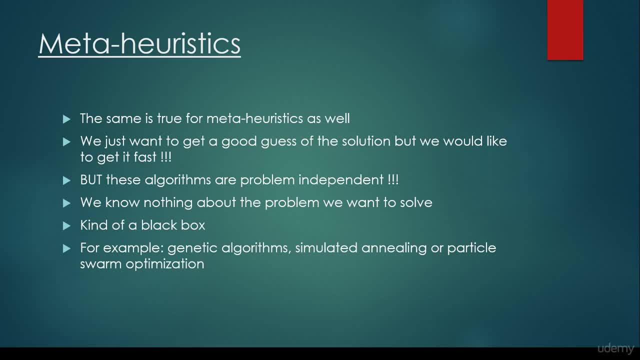 problems. Genetic algorithms can be used for solving the traveling salesman problem, But, for example, we are able to use genetic algorithms to calculate the edge weights for neural networks And basically, genetic algorithms are very, very important in this aspect. We usually 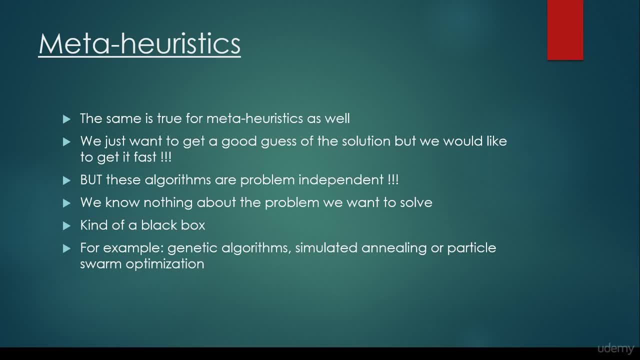 optimize and calculate the edge weights for neural networks with the help of genetic algorithms, And if the neural network is good, then we are able to approximate, for example, stock market values or we are able to recognize faces. Neural networks is a very, very important technology and algorithm. 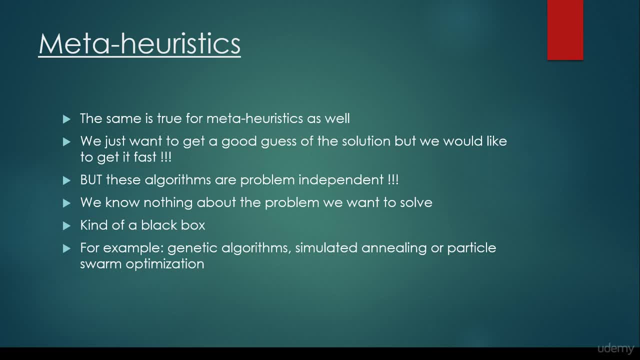 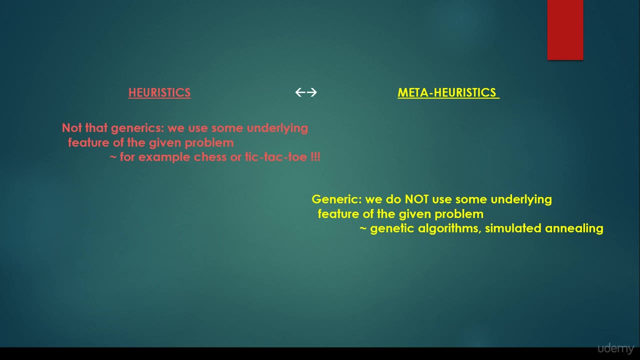 Most of the great companies relies heavily on neural networks, even in 2016,, such as Tesla, Google, Amazoncom and so on. So these meta-heuristics algorithms are quite important, and it's quite essential to see the difference between heuristics and meta-heuristics.